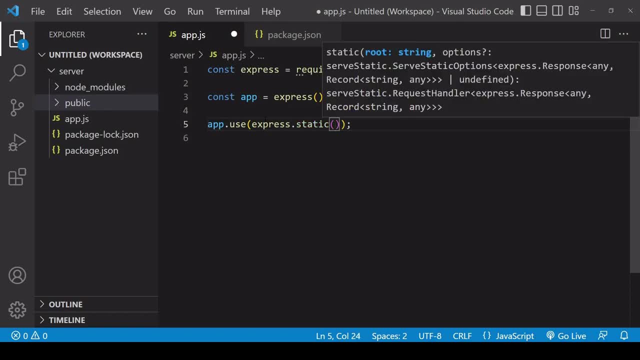 going to be doing is calling expressstatic, which allows you to specify a directory for serving static files. So in this case, if I enter public, then it's going to start serving files from the public folder statically when I start my app. So let's see this in action now by getting the app up and running locally on a report. So 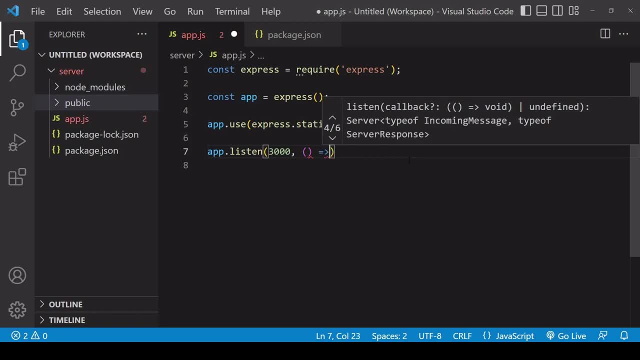 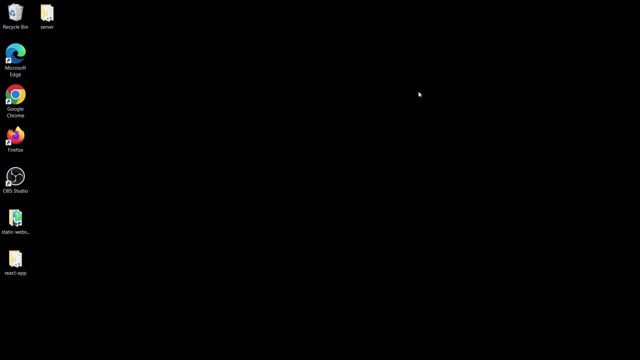 So let's see this in action now by getting the app up and running locally on a report. So usually port 3000 is a good port to use and I'll log something to the console here. listening on port 3000 now the public folder. it is still empty, so let's put something inside there. 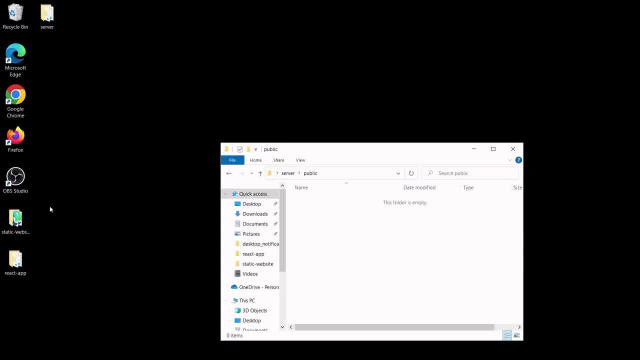 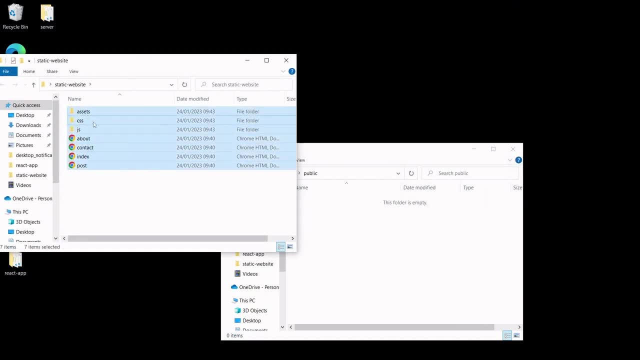 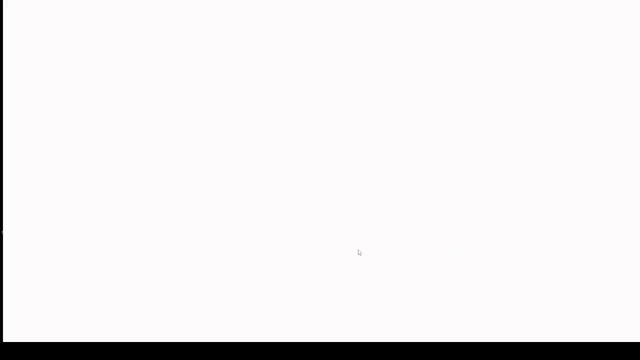 so I'll access the public folder here. and I have a basic html website here on my desktop, so I'm going to copy these files across and place them in the public folder. so I'll access indexhtml here so you know what it looks like. so it's a website template that I downloaded earlier. 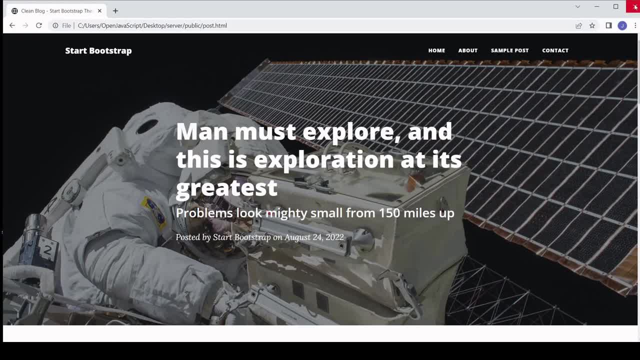 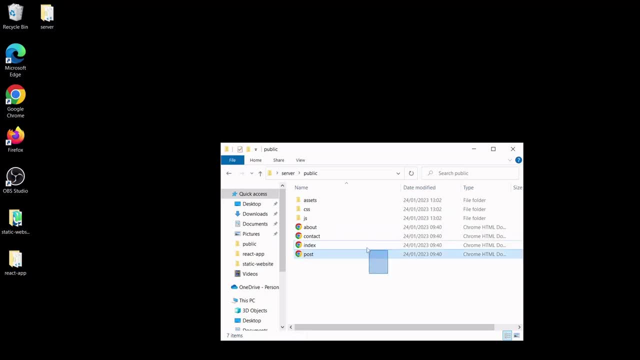 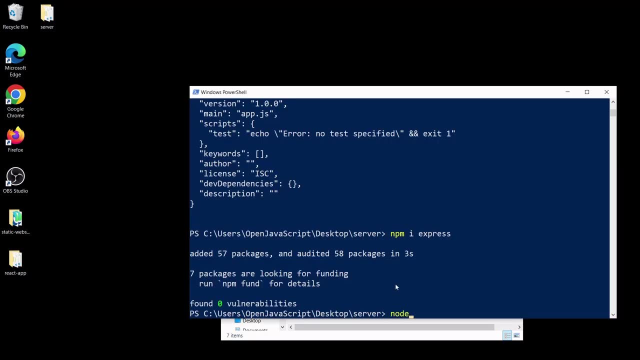 that is multi-page and, as you saw in the folder, it has some resources stored in subfolders that I needed to make the site work. so all of the content of this public folder is going to be made statically available when I start the server. so in my server folder I run node app, so it's telling me here that my app is now up and running on port. 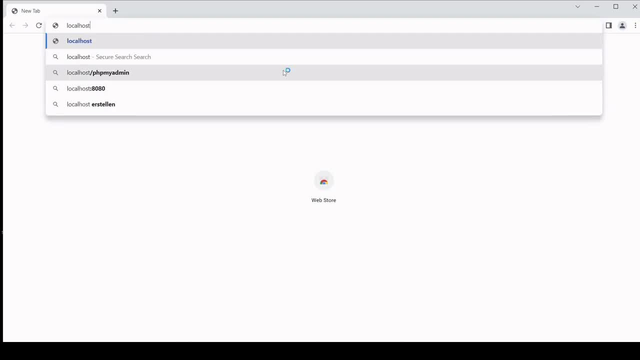 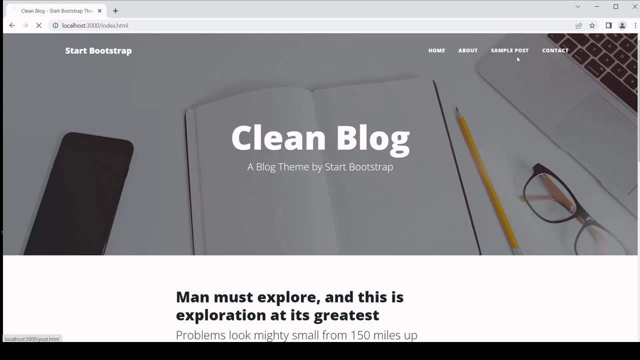 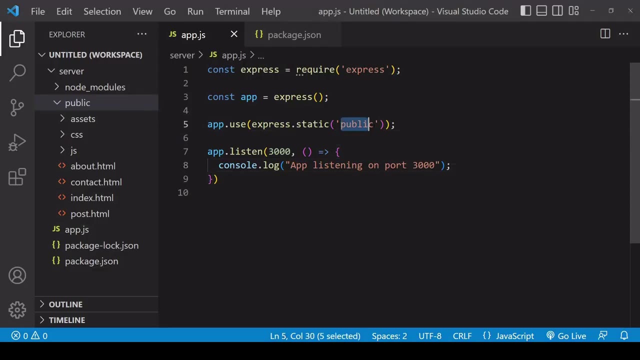 3000 and that's going to be on localhost. so if I access that port now, you see that the website is being served to us by the express app. now, although this is working, it's actually better practice to specify the path to the public folder a little differently from how I did it here. so initially, 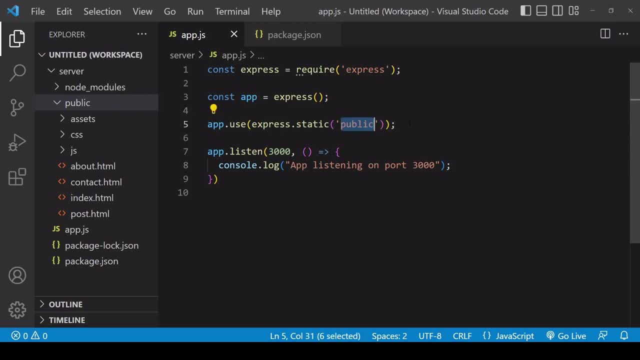 what I'm going to do that can come up here is that the public folder is relative to the working directory where I launched the app, not relative to appjs, even though they're usually the same. so you can get into a little trouble with this method. so if I try starting my app, one directory. 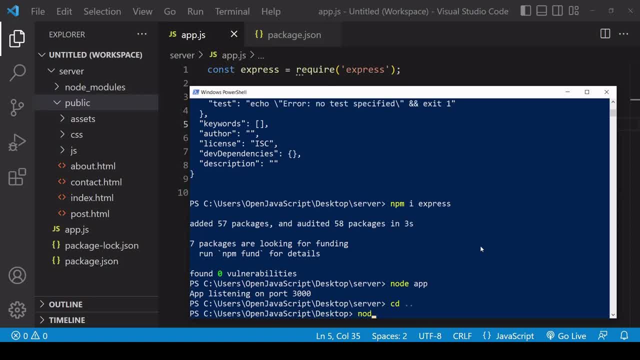 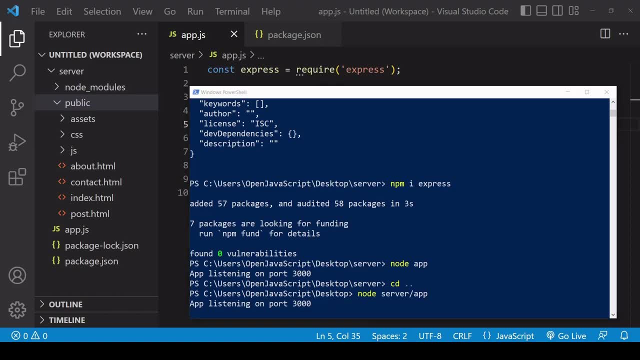 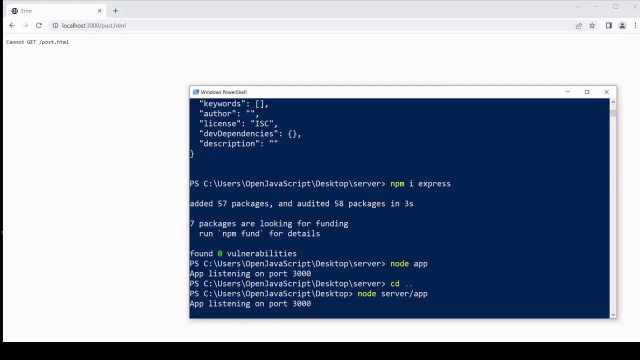 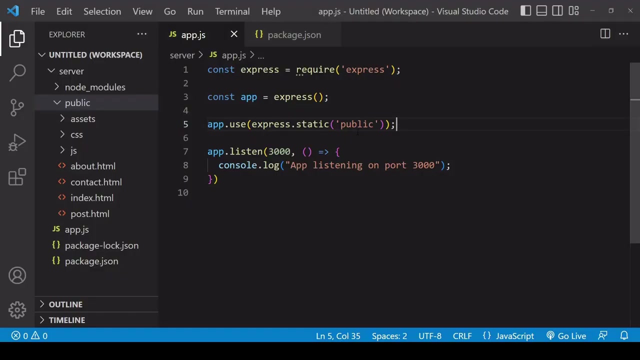 up from the server folder. so now I would start my app by running node server forward slash app. so that starts my app. but if I try to access it again, you see that the website cannot be accessed like before. the reason is that our working directory is now the desktop and there is no forward slash public folder on the desktop. 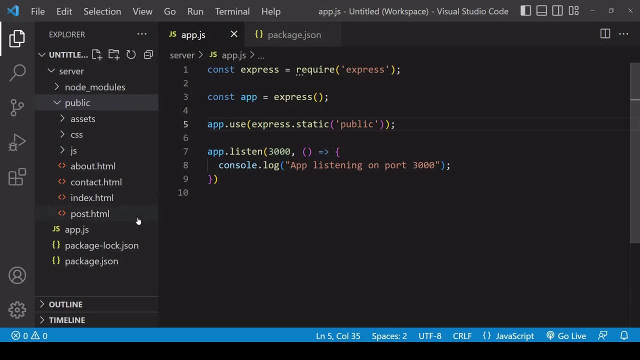 so to fix that we can set the path to the public folder relative to appjs and then, even if we start appjs from a different directory, then it's going to be able to find the public folder relative to appjs, so you can get the fixed path to the directory. 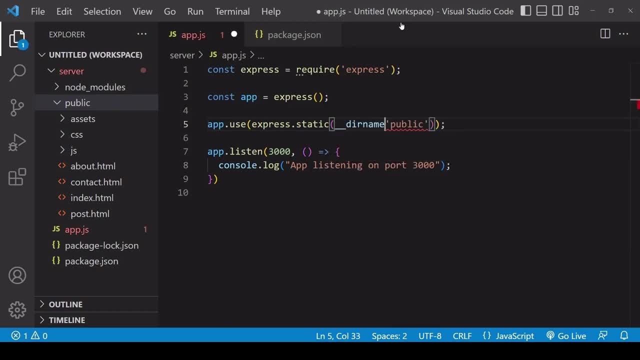 that contains this appjs file. by calling der name. now you could, if you wanted to concatenate the values here, to create the path, but it's actually better practice to rely on a core module for node here or path. so you don't need to do an npm install because this is already. 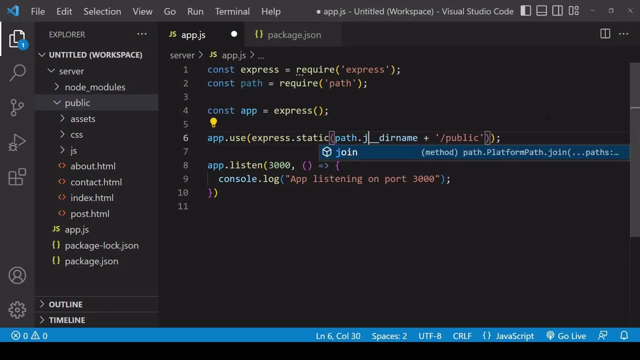 included in node, so you want to pass in the parts of the path into its join method as arguments. so the reason this is important is that you don't want to have to do that. if you want to do that it's useful is that when you're concatenating parts of a path, like we were before, you can. 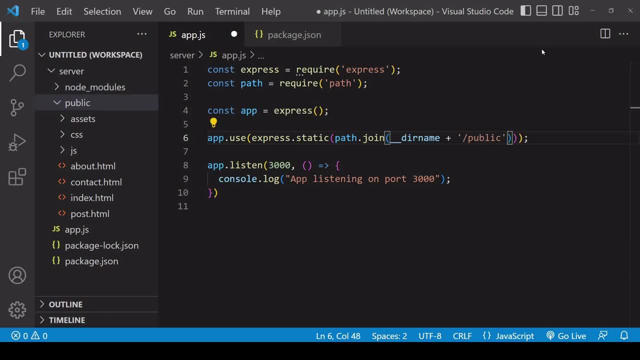 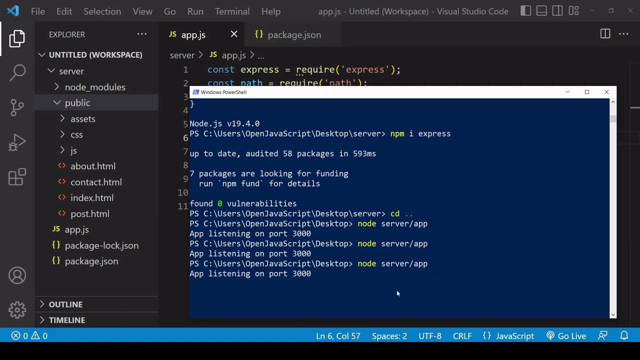 have problems with things like trailing slashes. using pathjoin is going to detect those issues and take care of those when you're creating a new path. so now, if we try to run this app again, one directory up from appjs, it should be working now, so let's try accessing the site. 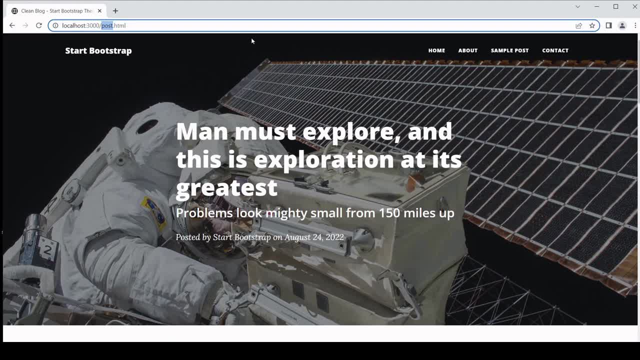 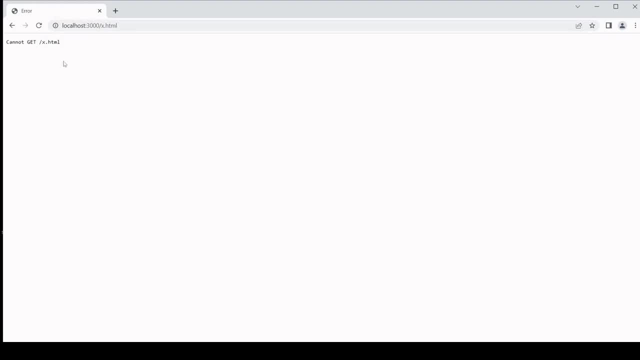 now, something you might want to add here is a 404 page, because if I try accessing a page that doesn't exist on the site, I get this message here. you might instead want to serve up a custom 404 message or a 404 page. so to do that call, appuse again. 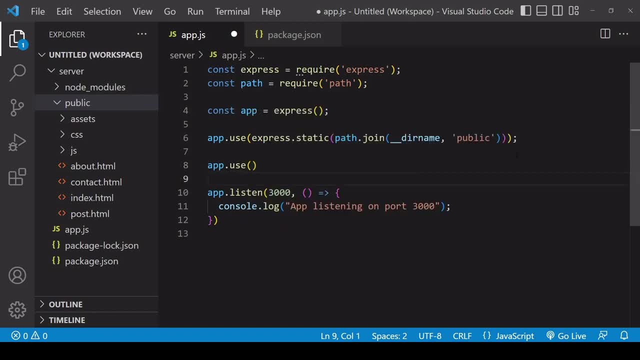 so after express has tried to serve up a static file. so if no resource that matches an incoming request is found in the public folder, then this appuse is going to run, and inside here what I'm going to do is to construct a response to the requester. so first I'm going to set a status code for response. 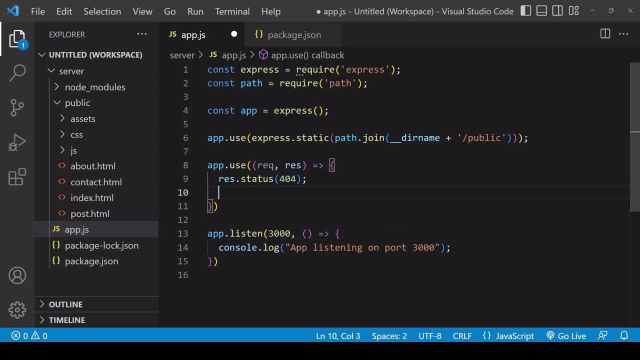 so I'm going to set that to 404 and then for the response itself, I'm going to specify some html here, so you could be sending a html document to the user here using send file and then specifying the path to the html document. but just for this example I'm going to be writing some html. 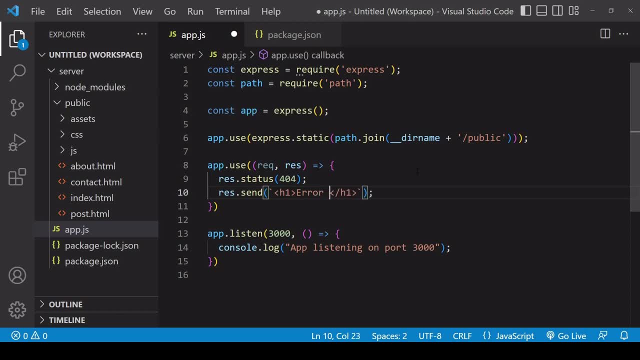 string, and then I'm going to be writing some html string, and then I'm going to be writing some html- ival ME singer, and then I'm going to be-. so progress will now say: professional error be traps, and it's going to want it as a強 reference for me to browse I can't access. 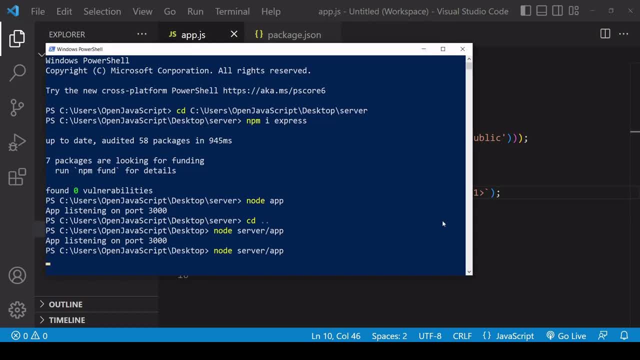 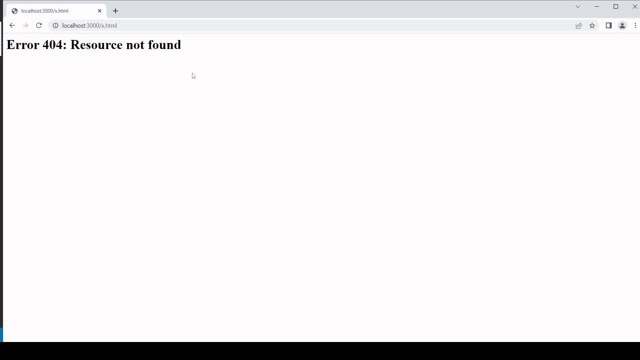 it myself, and now the full info that I will get from the reseller bin is going to be code register code again. this tells me that server isn't a transport explicitly. I can't access it from the public folder, they just get it from the public folder. so so this is what I want. 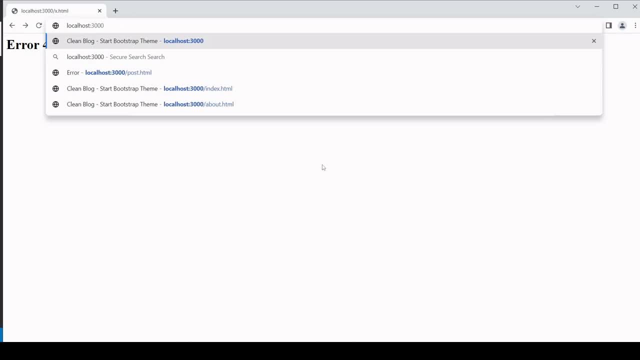 we can 내 서명. 보면도 볼 수 있는데 benefic, debut, 대박 letters. Lakewood is totally off the radar. I'm going to go to the email representative. that is on port 3000 on localhost. so quite often this is what you want, but if you do find yourself, 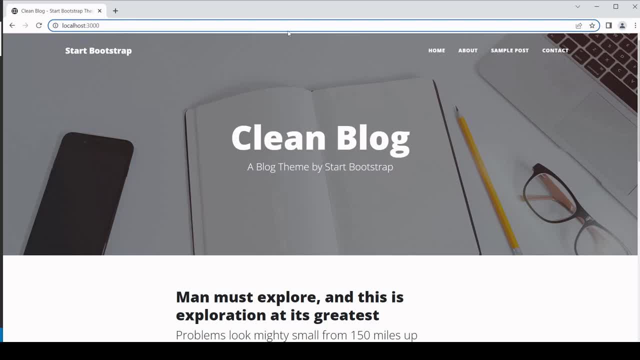 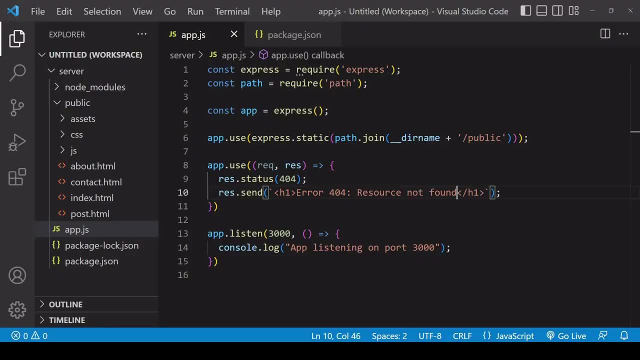 wanting to serve your content on a subdirectory of the root, such as forward slash website here, then what you can do is, in appjs, simply specify a path as a first argument inside appuse. so, relative to the root, I'll specify here forward slash website. now, when I restart my server, 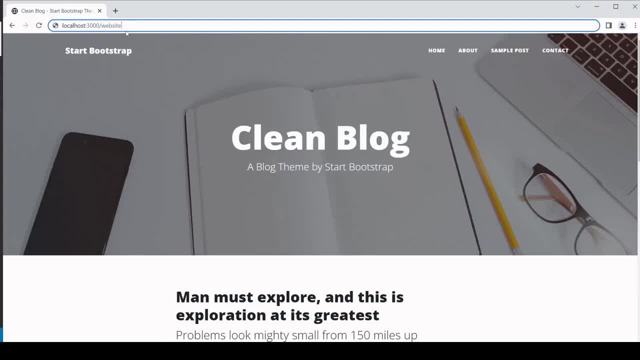 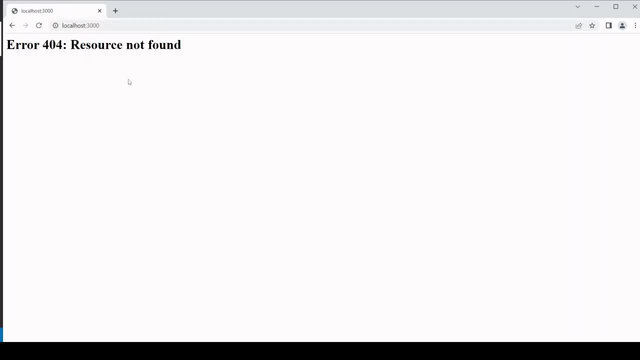 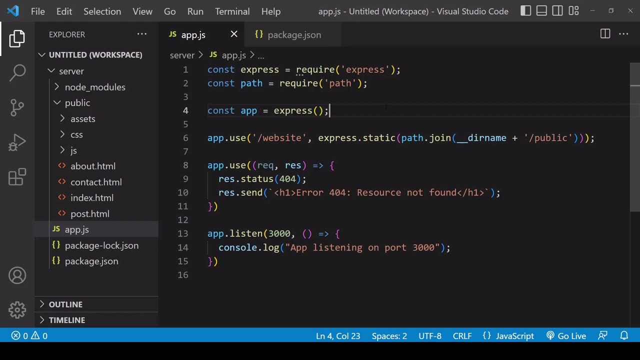 and I access localhost 3000 forward slash website. the website is now being served there and if I go to the root you see that there's nothing there now. so I won't change the path on which the website is being served back to root, because I want to keep that free so I can show you. 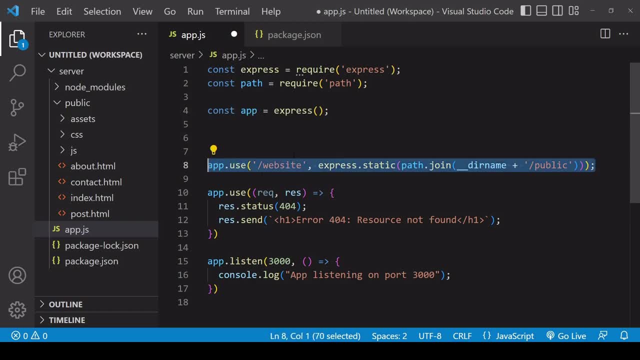 now how to serve a react app. so I'm going to copy the syntax that I use to specify a public folder. I'm going to specify another public folder, so I'm going to store my react application in a folder called react app on the server and I want that to be served up when a user makes a request to the root. now I do already have a react. 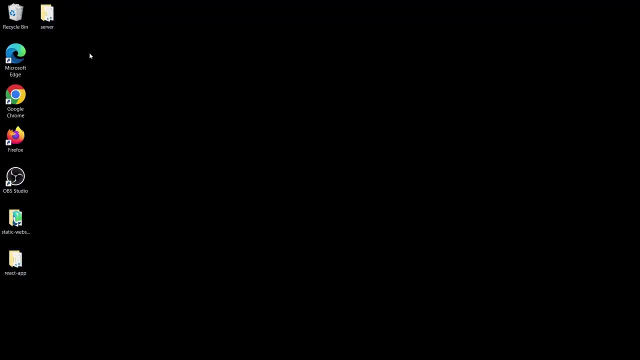 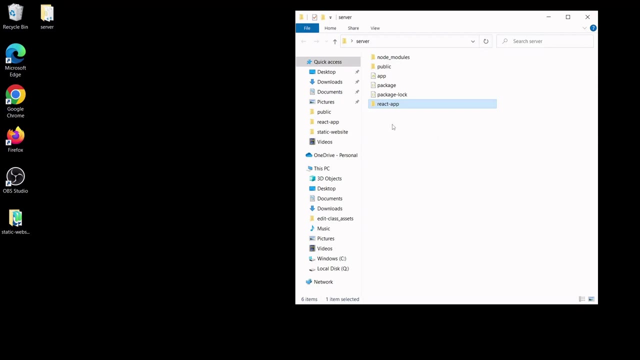 app sitting on my desktop here that I created earlier. so what I'm going to do is to drag and drop that into the server folder and I'm going to copy that into the root and I'm going to save it as a public folder. now I don't need to make any changes to the server side path yet. 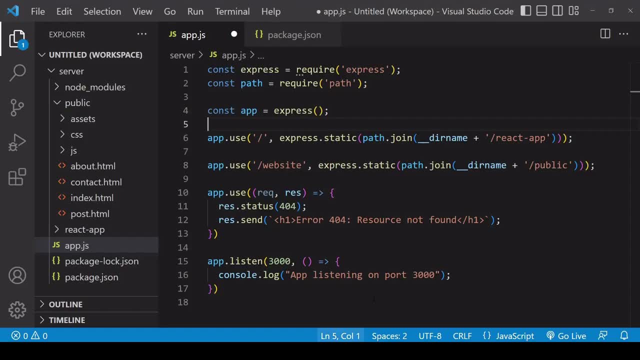 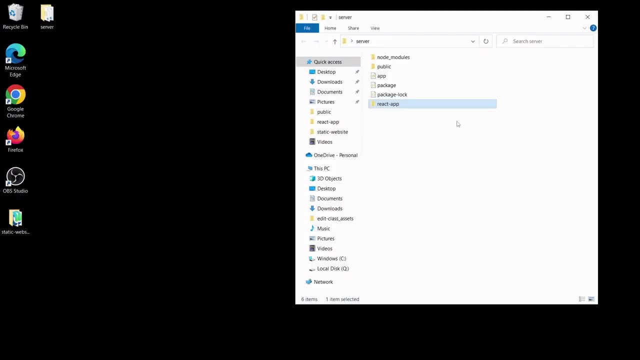 because the folder here is called react hyphen app and inside appjs. I'm serving up on the root contents of the folder react hyphen app at the react app folder. it just contains the contents of a new react app that cannot be served statically. so what you need to do to be able to 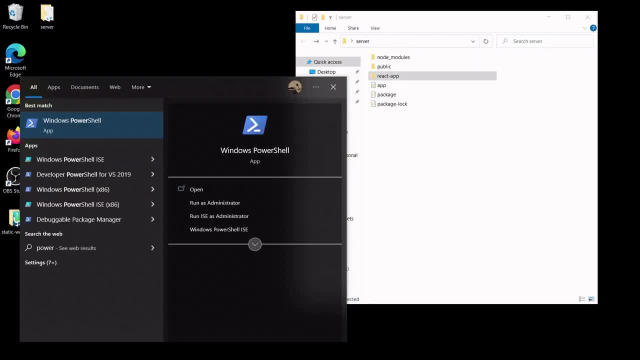 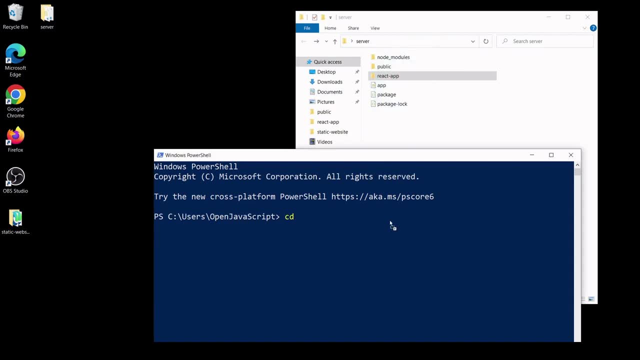 serve it statically is to create a production build of your react app. so to be able to serve that, I'm going to first of all cd into the react app folder. so if you use create react app, you create the app like I did. then you can run here npm, run build and this is going to create. 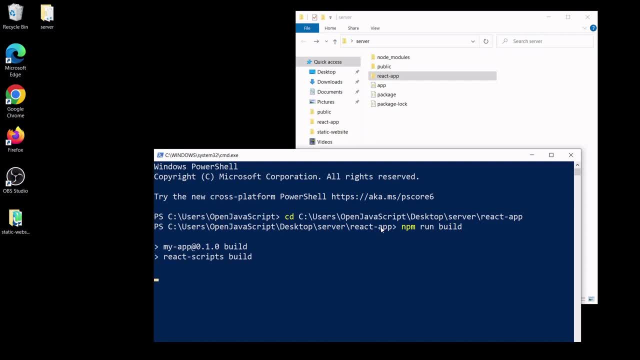 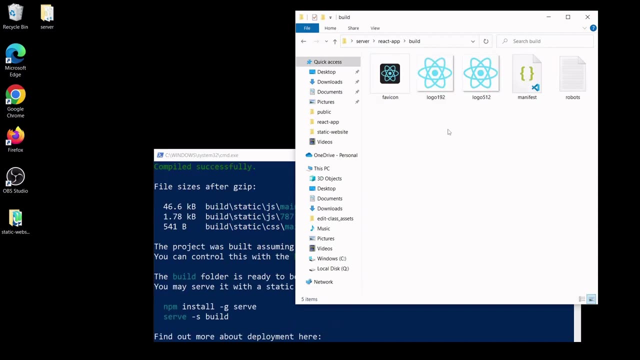 a production version of your app that you can host statically, and it's going to do that by creating a new folder inside of react app that's going to be called build. okay, so now that it's there, your react app ready to be served, it's inside the server, inside react. 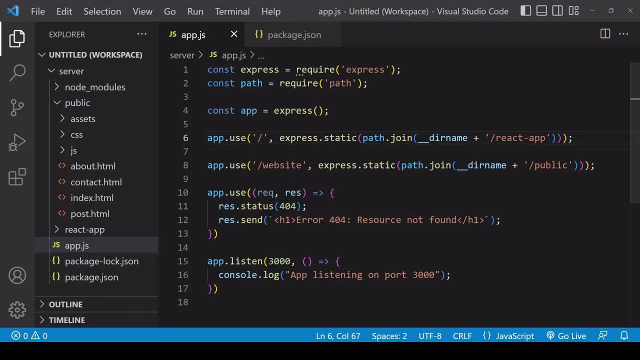 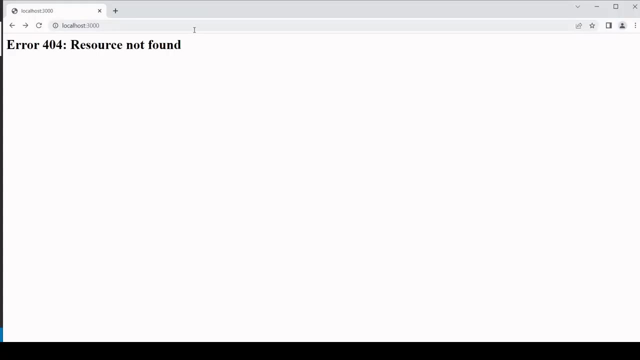 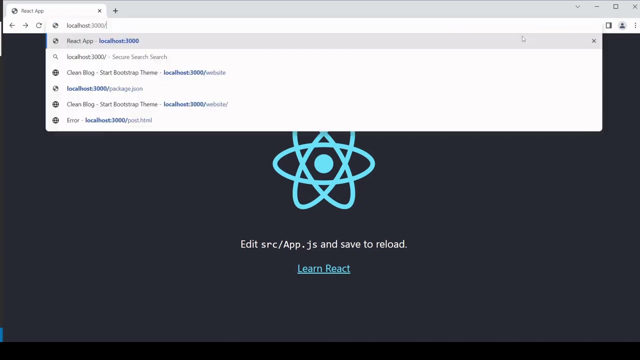 app folder inside the build folder now. so you need to add forward slash build to the server side path. now if I save this and I restart my server and access the root, hopefully the react app it's now being served on the root. and if I access the root forward slash website,